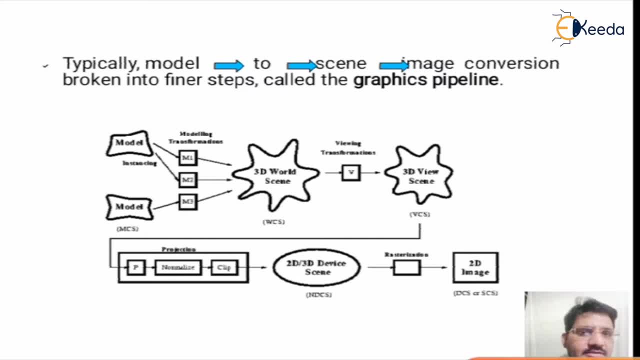 pipeline. we can see the process in diagram. First any model convert in world coordinate system. that is, first model convert in 3D scene, then when we apply viewing transformation on 3D scene, then the world scene convert in view coordinate system, which is called view coordinate system, but again it is in. 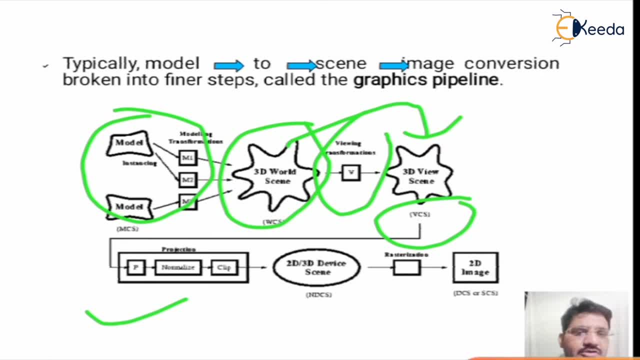 3D platform. So we apply different projections, normalization and clipping approach. then this images convert in required normalized coordinate system. It may be on 2D or 3D, After applying rasterization, the normal device coordinate system, which may be in 2D or 3D. 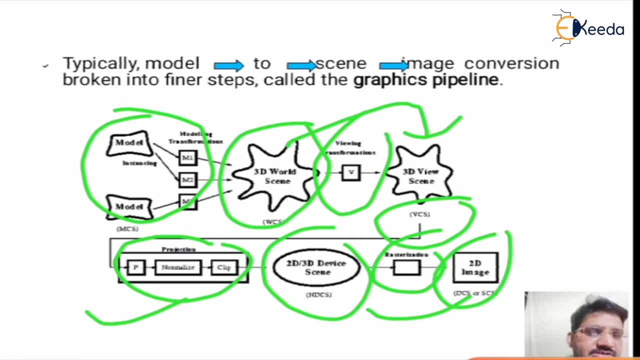 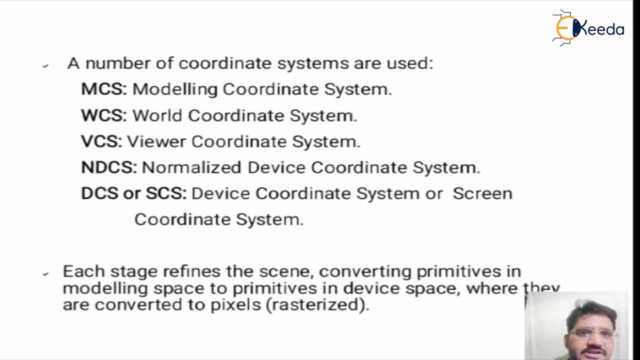 convert in 2D image coordinate system, which is a device coordinate system. During rendering pipeline we can use different coordinate systems like modeling world coordinate, viewer coordinate, normalized device coordinate and device coordinate system or screen coordinate system. In each stage we refine the scene and convert. 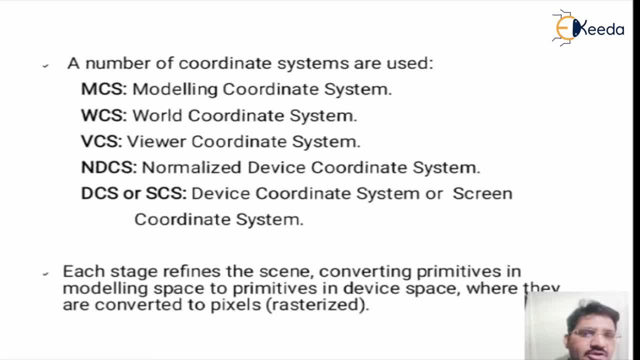 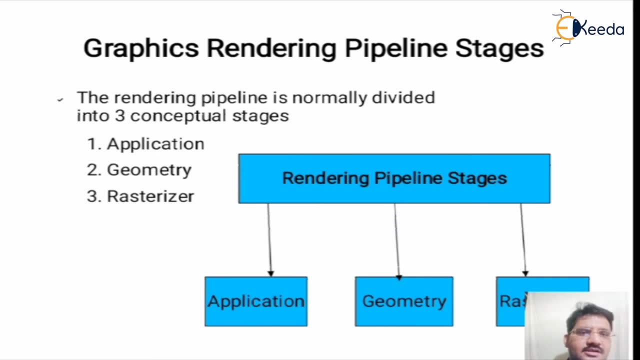 the object in modeling space to primitive in device space, where they converted in pixel or rasterized form. There are three stages in rendering pipeline. First is application, second geometry and third is rasterizer stage. Let's see about all these three In the application stage. 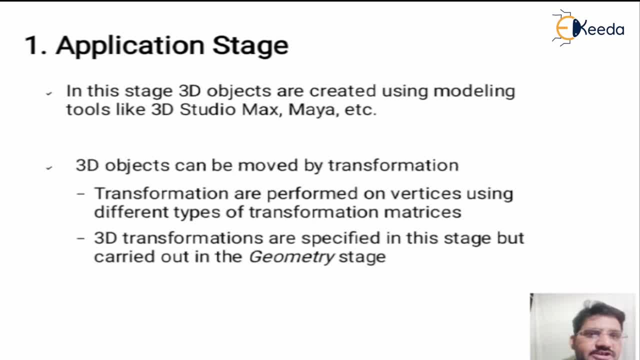 3D objects are created using different modeling tools. for this we can use 3D studio, max, Maya and other application software for this purpose. 3D objects can be moved by transformations. The transformations are performed on vertices using different type of transformation matrices. 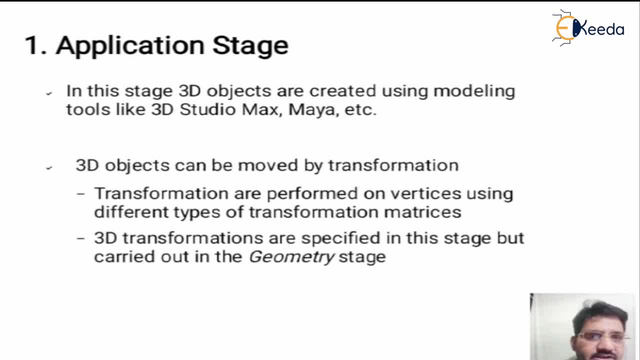 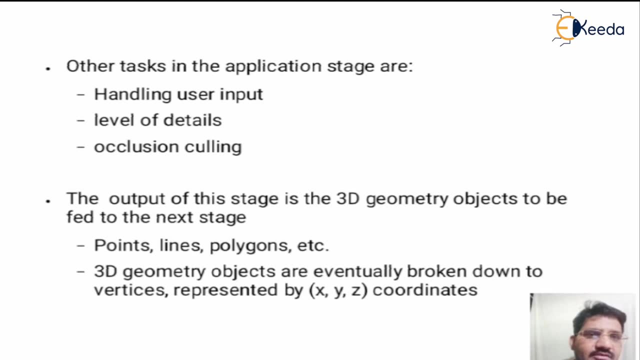 The 3D transformations are specified in this stage, but we use the output of this stage in geometry stage, which is next stage. Other tasks of application stage are handling user input, levels of details, occlusion, cooling. The output of this stage is 3D geometric object. 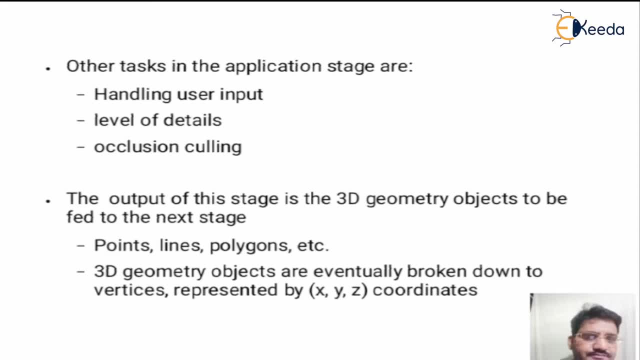 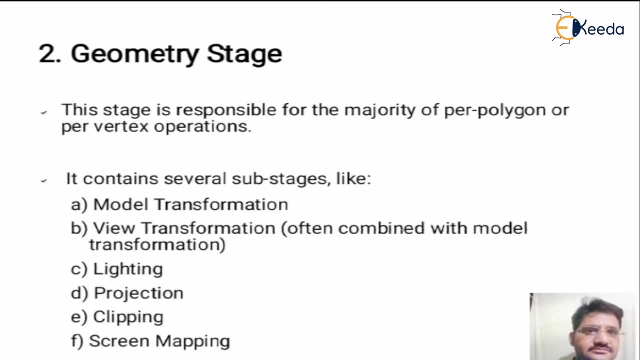 which use as input. The outputs are, for this stage, points, lines, polygons, which are used as input for the next stage. The second stage is geometry stage. In this stage we are responsible for majority of per polygon or per vertex operations. This stage can be further. 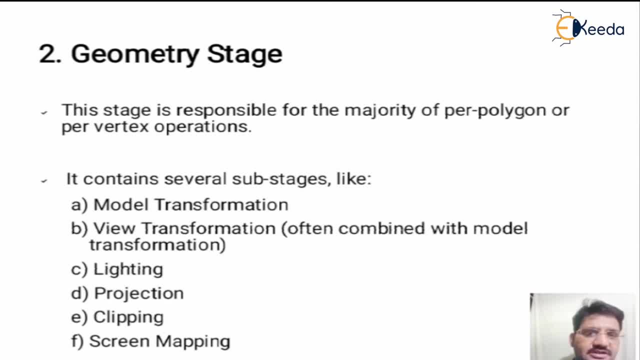 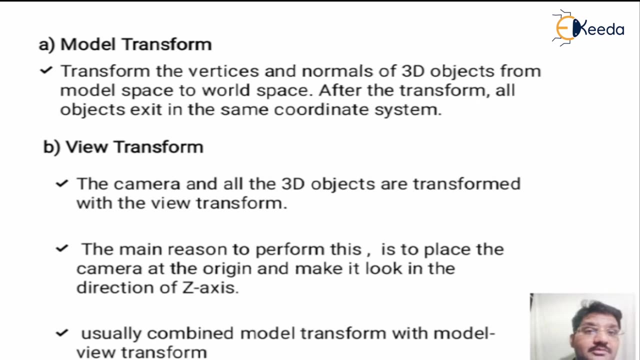 divide in sub stages or it contain the following sub stages, like model transformation, view transformation, lightning projection, clipping and screen mapping. In brief, model transform, model transform: transform the vertices and normals of 3D object from model space to world space. After this transformation: 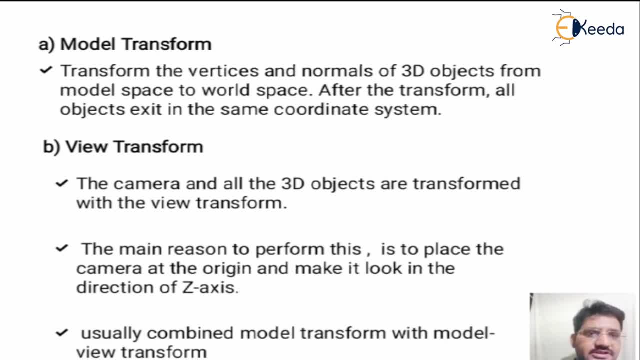 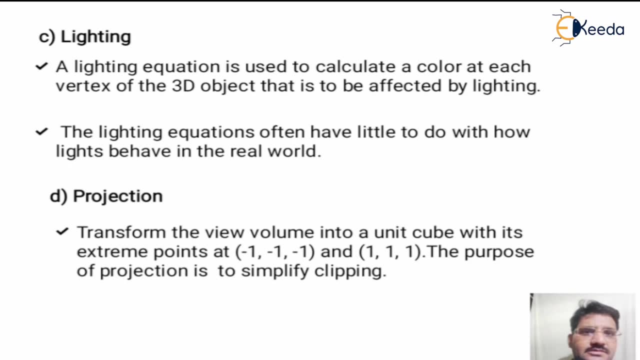 all objects exit in the same coordinate system In the view transform camera and all the 3D objects are transformed with the view transform. Usually we combine model transform with the model view transform. In the lightning a lightning equation is used to calculate a color at each vertex of the 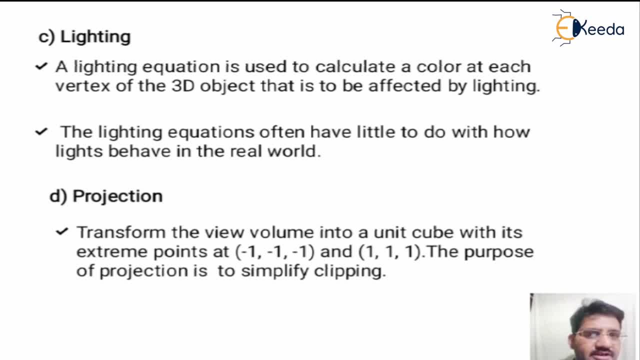 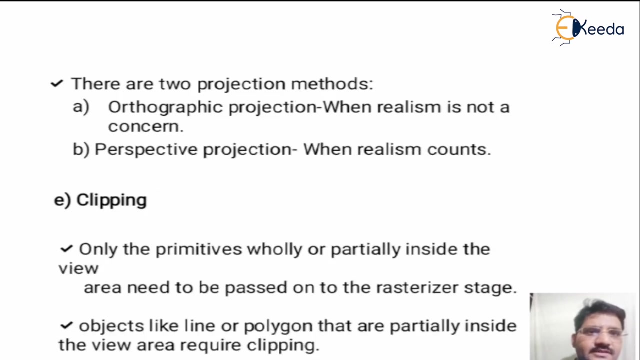 3D object that is to be affected by the lightning In the projection. transform the view volume into unit Q with its extreme points at and, and. The main purpose of projection is to simplify the clipping. Projection can be done by two methods: orthographic, that is when 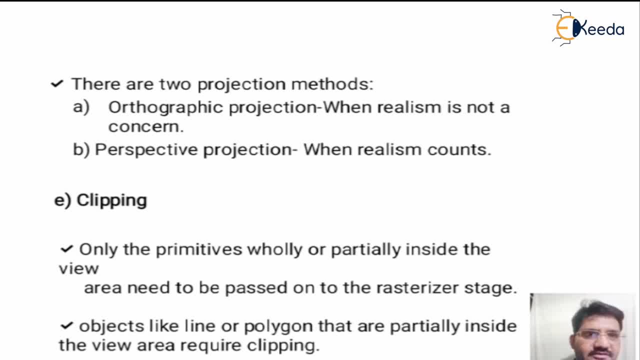 realism is not a concern and perspective when we focus about realism After projection clipping done In the clipping, only primitives which are completely or partially inside the view are needed to be passed on to the restoration stage and the object, like line or polygon that are partially inside. 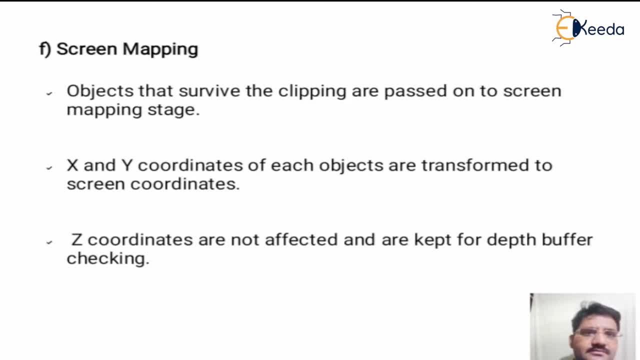 the view area required for that clip In the screen mapping. objects that survive the clipping are passed on the screen mapping step. X and Y coordinates of each objects are transformed to screen coordinates and the Z coordinates are not affected And we keep information of Z coordinates. 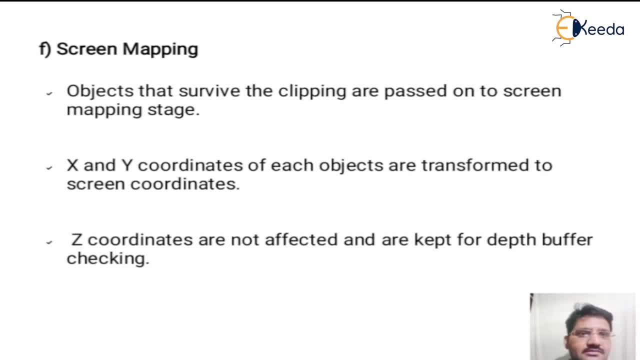 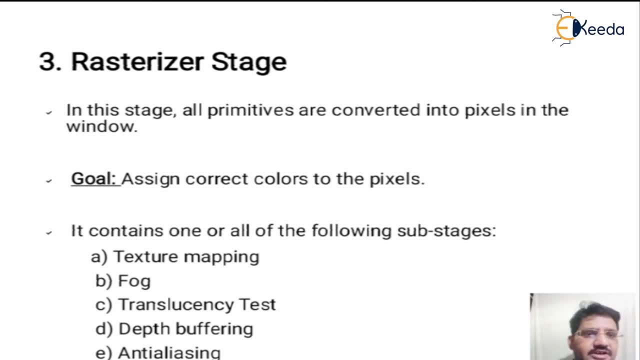 in depth buffer or Z buffer. In the third stage, restoration stage. In this stage, all primitives are converted into pixels in the window. The main goal of this stage is to assign the correct colors to the pixels, and this stage consists the following some stages: 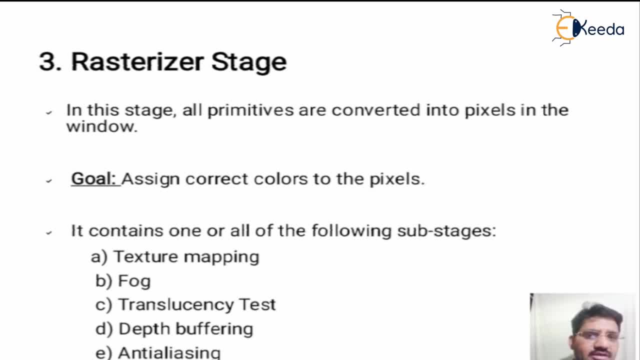 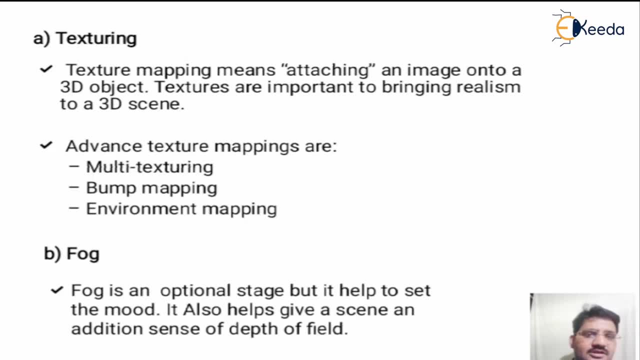 like texture mapping, fog transparency, test, depth buffering, anti-aliasing. Discuss in brief all about these. First is texturing. Texturing means attaching an image on to a 3D object. This is a texturing mapping, and textures are important to bring realistic 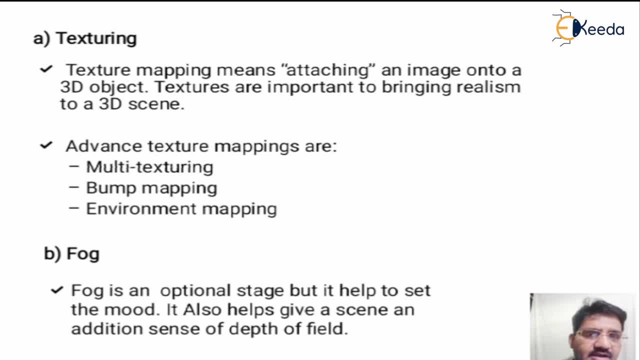 realism effect in a 3D scene. Advanced texture mappings are multi-texturing bump mapping, environment mapping, which we will discuss in later videos In the fog. it is an optional stage, It's not compulsory, But it helps to set the mood. It also helps give